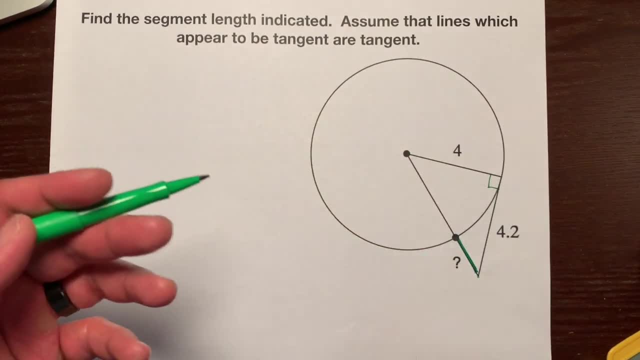 This is the question mark. when we have a right triangle And we have at least information about two sides, We can use the Pythagorean Theorem. So let's use the Pythagorean Theorem. Remember the Pythagorean Theorem is c: squared is equal to. 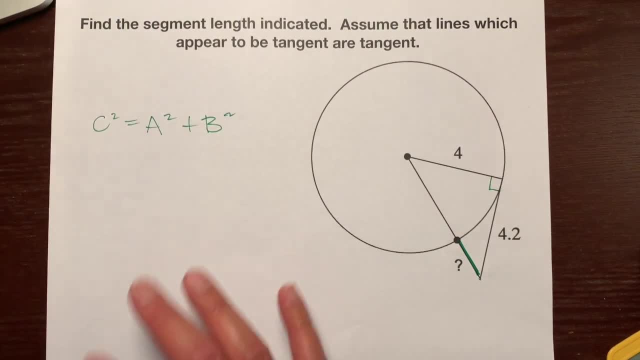 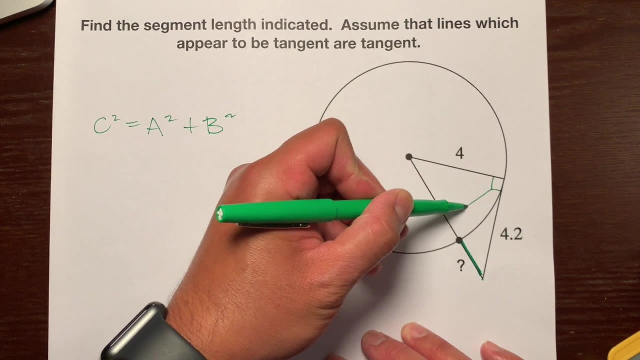 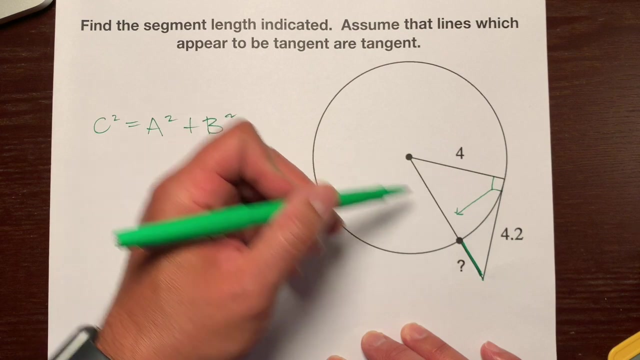 a squared plus b squared and the c is the hypotenuse. the hypotenuse is the side that is opposite. the right angle, here's the right angle and it's looking at the hypotenuse right there. so this entire side right here is the hypotenuse. uh, we're trying to just find this, but what's the? 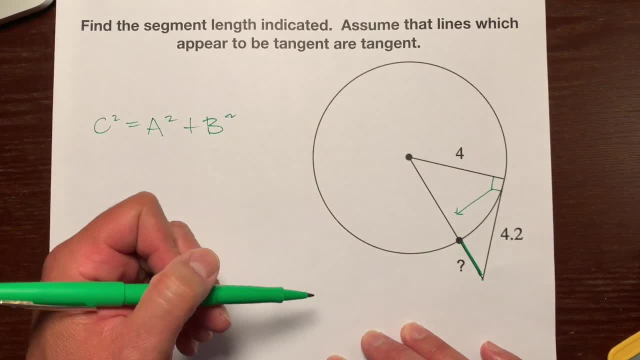 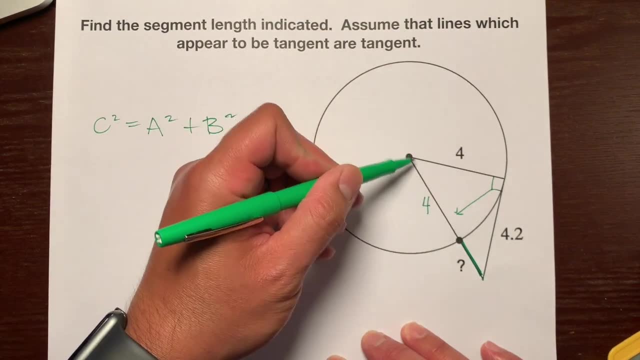 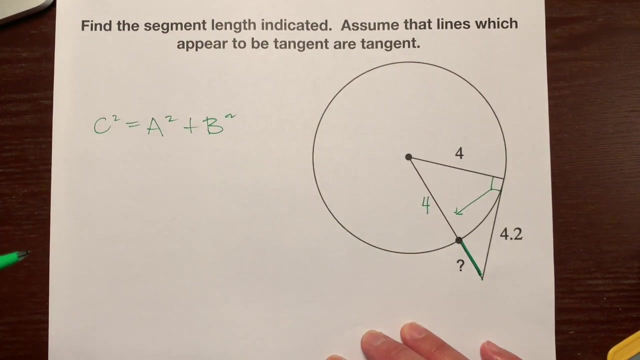 length of this right here. do we have any information about this whole thing right here? um, yeah, so the length from here to here is four, because that's the radius. so the length of this our information about c is four plus question mark. um, so the hypotenuse that we have is, uh, four. 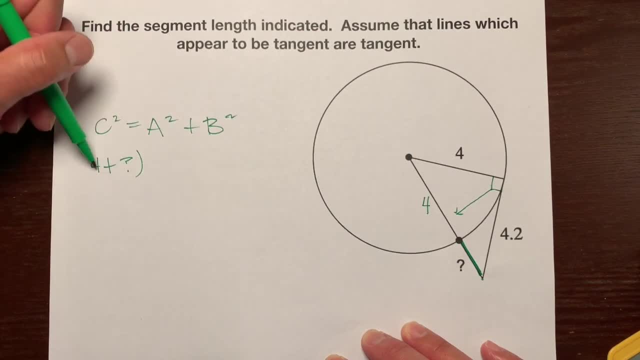 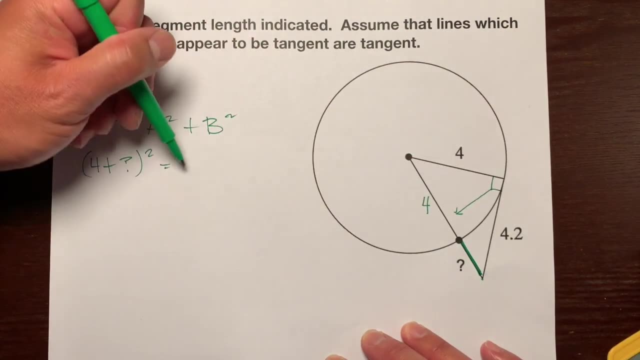 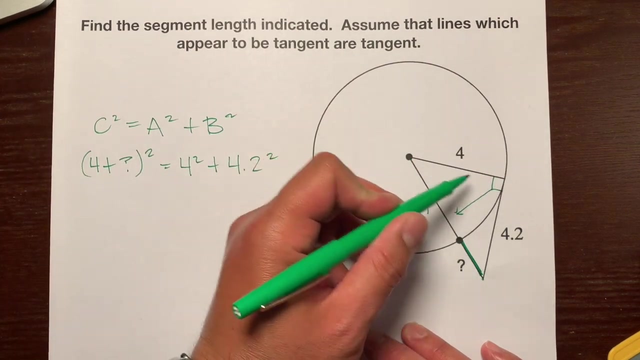 plus question mark squared. so this is our c right here, and we'll set it equal to uh a squared, which is four squared plus 4.2 squared. so here's our a, here's our b, or this could have been your a, this could have been your b, doesn't matter. and then let's just grab our. 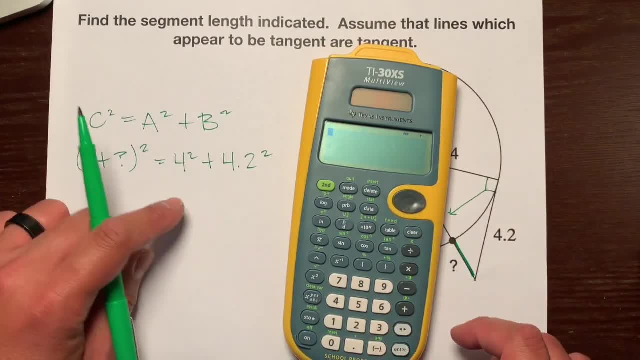 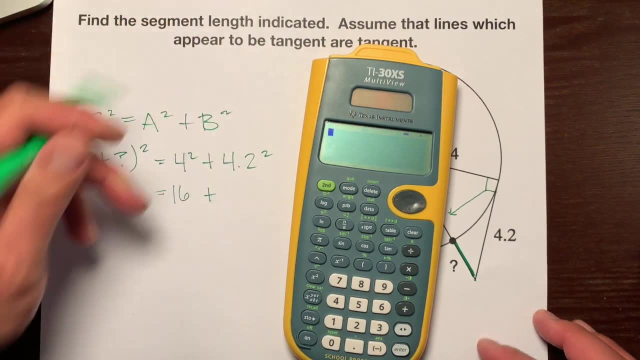 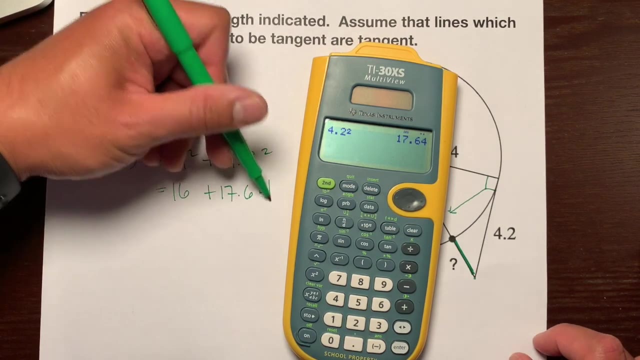 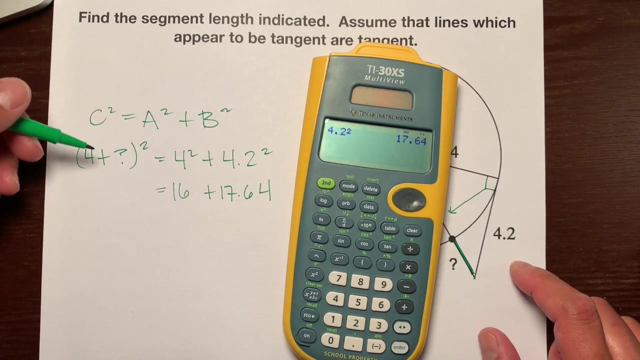 calculator and start scoring some numbers. so four squared? well, we don't need a calculator for that, hopefully not. four squared is not eight, it's 16. but what's this decimal square? so 4.2 squared is 17.. six four is equal to. so now, here you're going to be tempted to do some algebra. definitely don't. 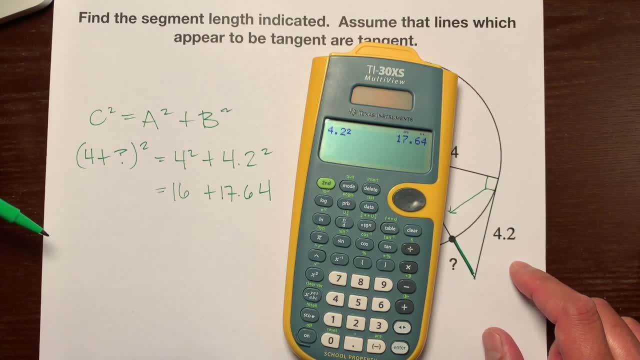 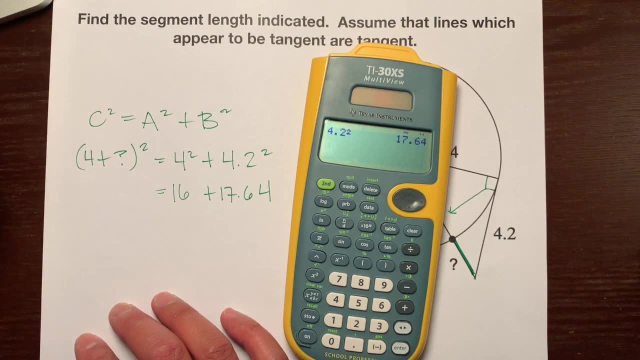 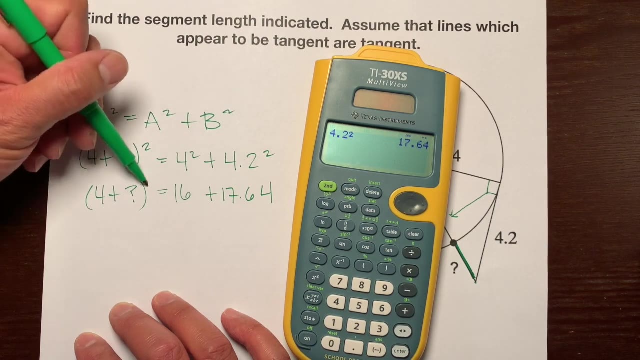 be tempted to distribute the square here and here, because that's against algebra rules. um, you'll be tempted to. um might write four plus question mark times, four plus question mark, because that's real algebra. uh, but don't do that, so just bring this down, okay, and let's combine these two like terms.